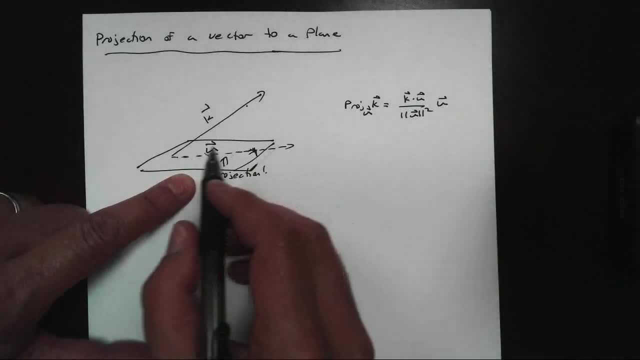 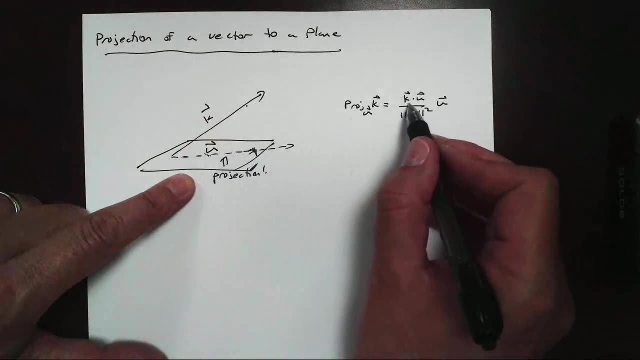 The problem is we don't know what u is See. earlier we could find it because we did the projection of a vector onto a line, So I could easily. if I'm given the line I can get that projection. But if we don't have that line it gets a little more tricky for us. 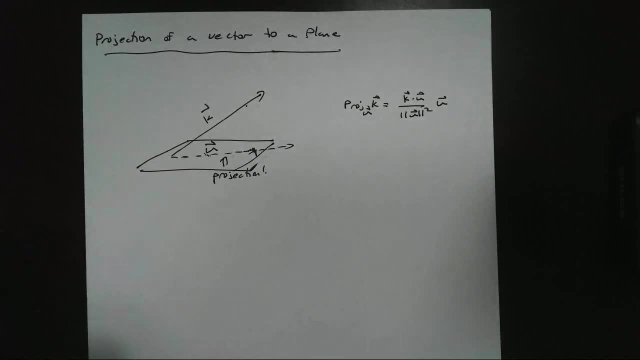 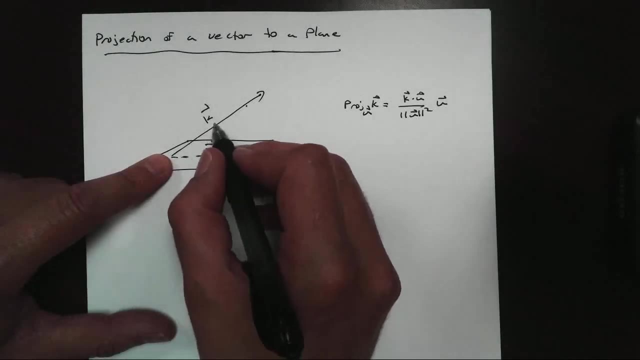 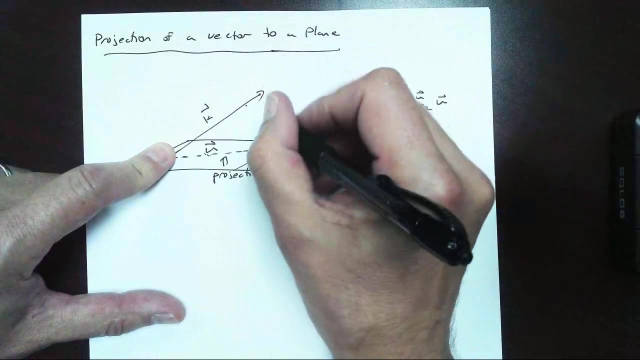 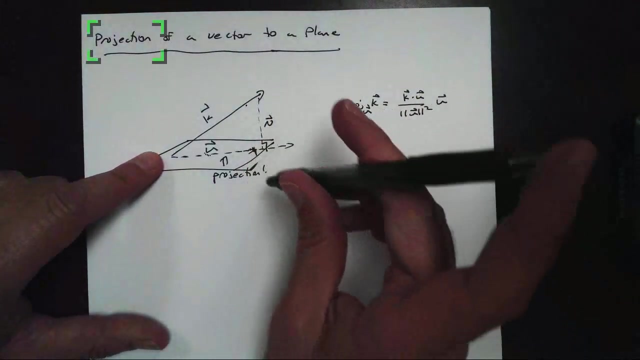 So we're going to kind of go about solving this another way. What we do instead is: we're not going to find the projection of k onto u, we're going to find the projection of k onto the normal vector. So because any there's my normal vector, we'll call it n for normal, because any normal vector is always going to be perpendicular to the plane. 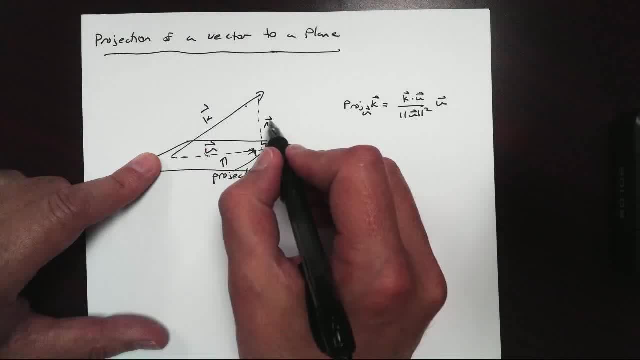 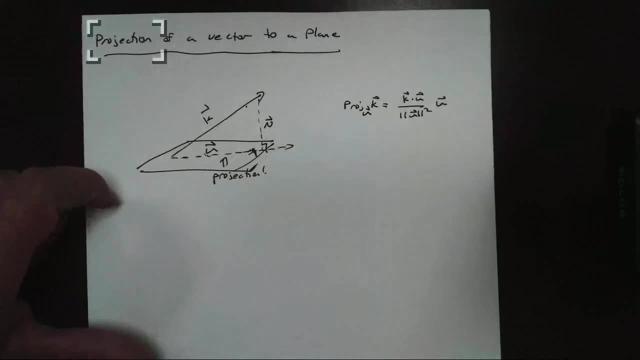 And we're going to use that idea. So, and this one, I do know We will know the equation of the normal vector Because this comes from the equation of the plane. We'll get back to that again in a little bit. 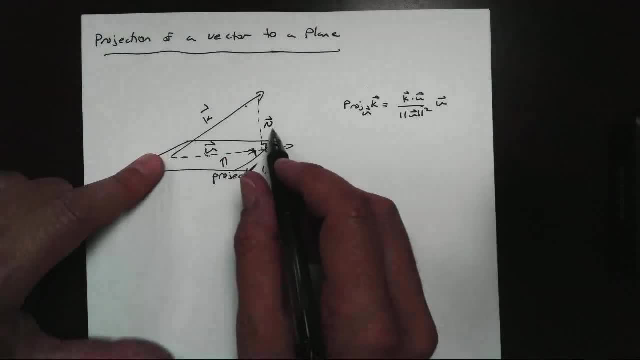 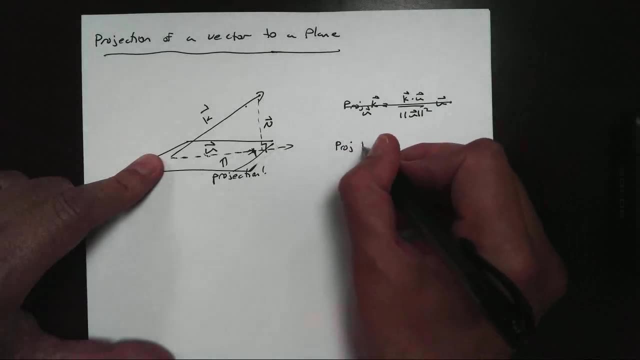 And there's also another video on that. Smash that like button. So what we're going to do instead? since I can't find this? instead, we're going to look for the projection of k onto the normal vector, And that's what we're going to do here. 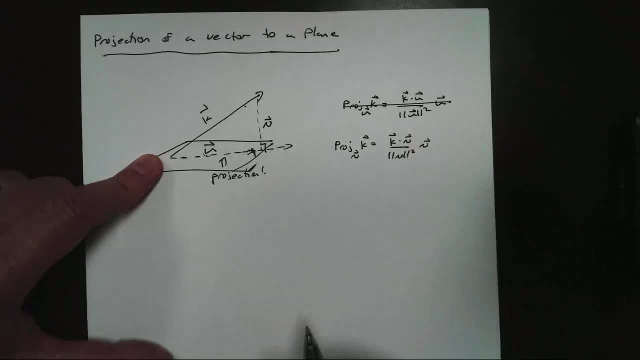 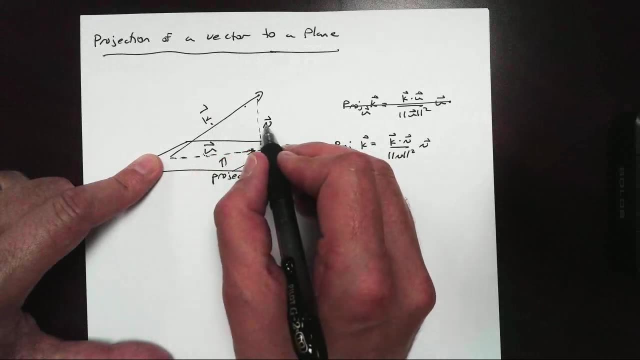 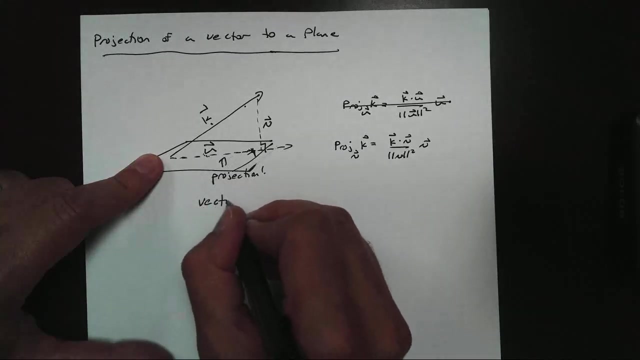 And let's talk about why we do this. Well, if I know k and I do know n and I'm looking for the projection here ready- That I could use vector addition to solve whoops addition, there we go. 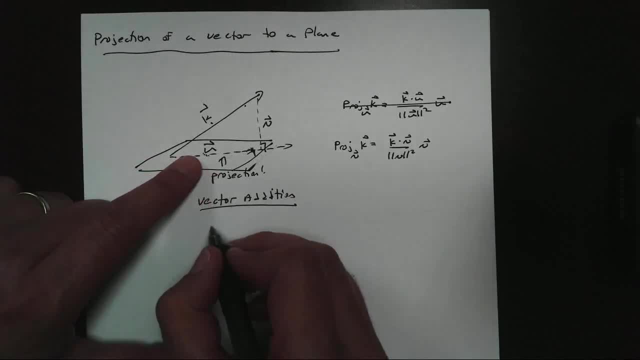 So I'm majoring in math. I can use vector addition to solve for the projection I want, For example, because I know u plus n has to equal k And I can solve for it. u, which is the projection I do want, will equal the vector k. 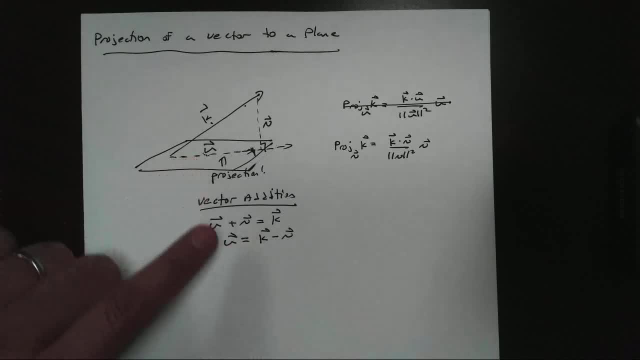 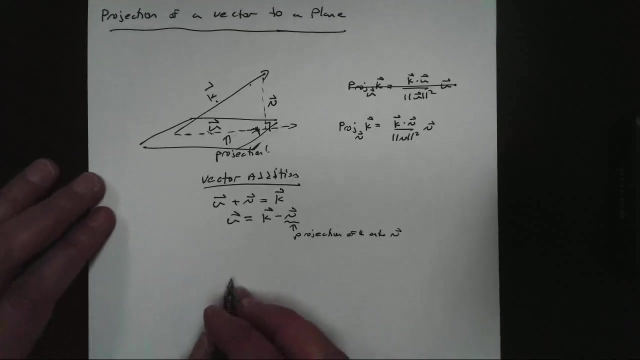 minus my normal vector. Okay, But remember, this really isn't the normal vector. This is really the projection of k onto n. So let's go ahead and get started with this. So let's say, we have a plane here. 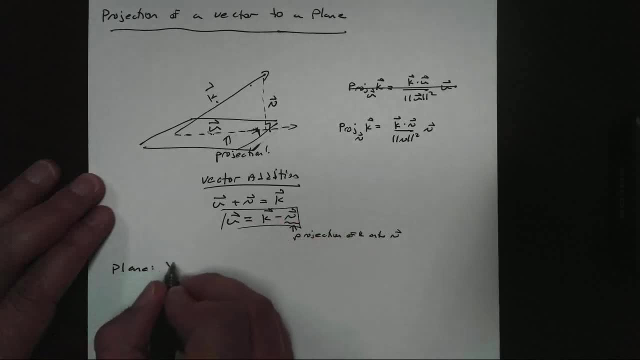 So this is what I'm looking for eventually. Let's say we have a plane that's given by the equation x plus z equals 3.. And we have vector k, which is given by 1,, 1, 1.. And what we want to do is: 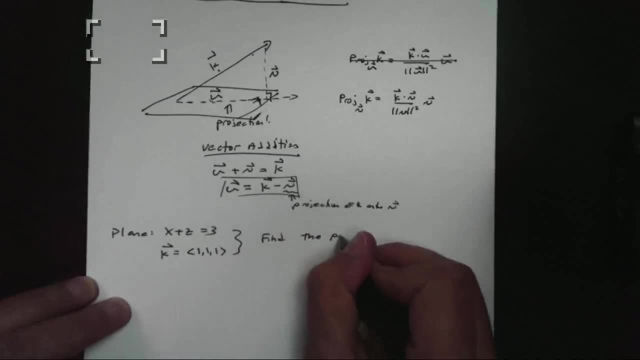 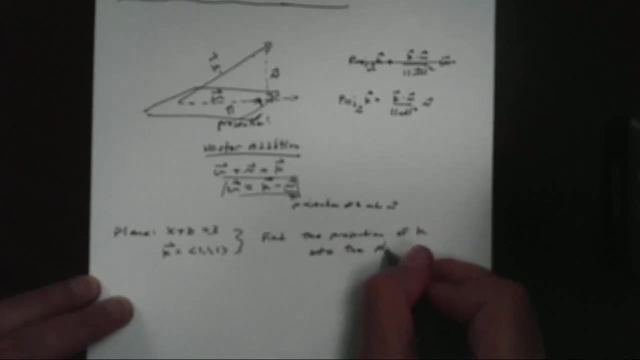 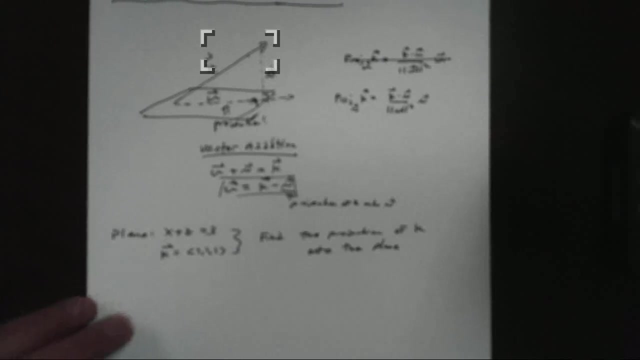 we want to find the projection of k onto the plane. Now, I don't know, I got a little out of focus there, Sorry about that, So let me go ahead and fix that real quick. So what we want to do is: 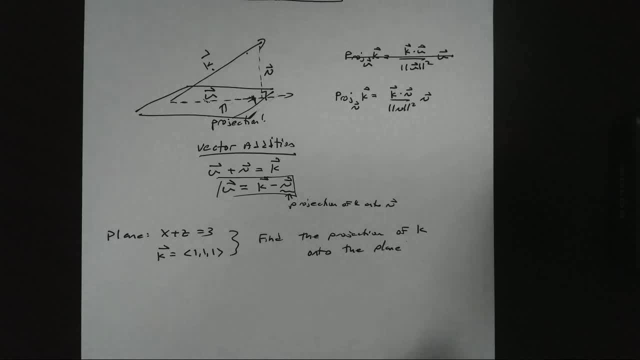 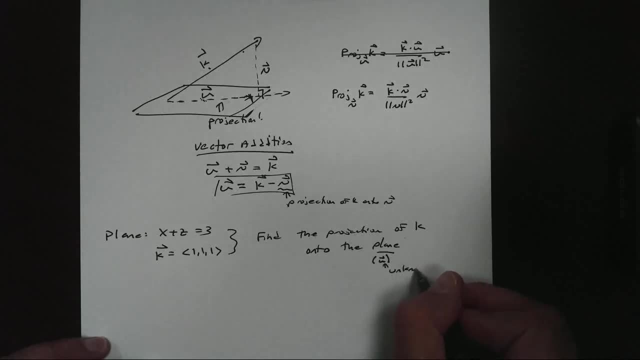 we want to find the projection of k onto the plane. Now again, the big problem is the plane here is being represented by u, which is unknown, So I can't go about finding it directly. If I think about vector, u is the line on the plane. 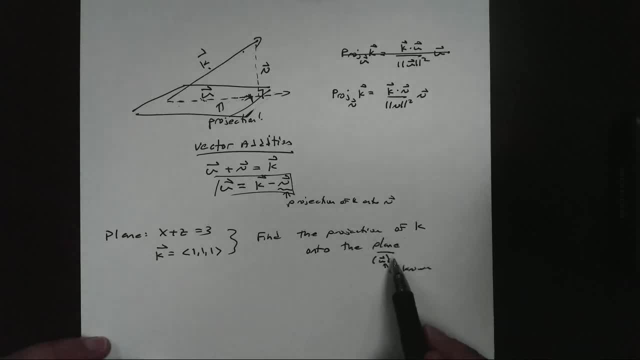 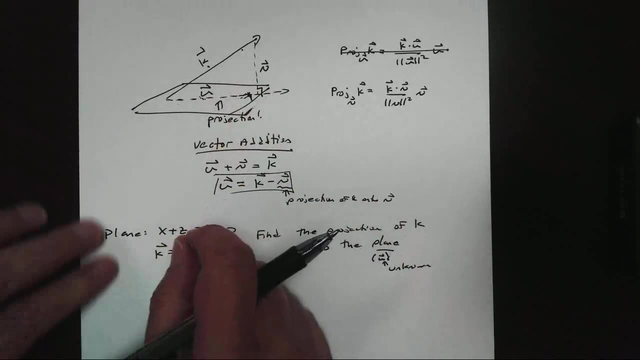 of the projection that we're wanting, but we don't know it. So what we're going to do first is we're going to find the projection of k onto our normal vector, And that's because no matter where our normal vector is. 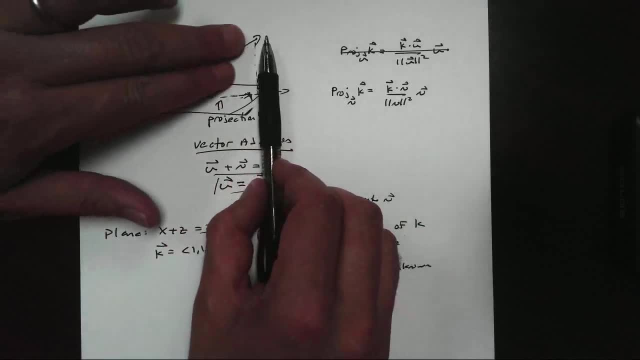 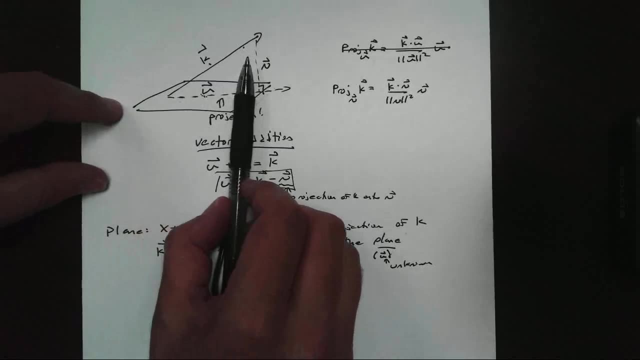 right here. if I shine a light coming in this direction, that shadow length will never change, even if I put it way over here. If I put it over here, the light coming down this way, the length of our projection for n will never change. 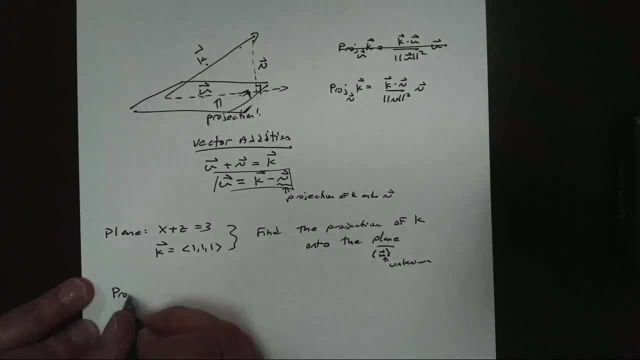 So we can do that. We're going to find the projection of k onto n first, And to do this, let's write out everything we know. Okay, to do this we need vector k, which we know is 1, 1, 1.. 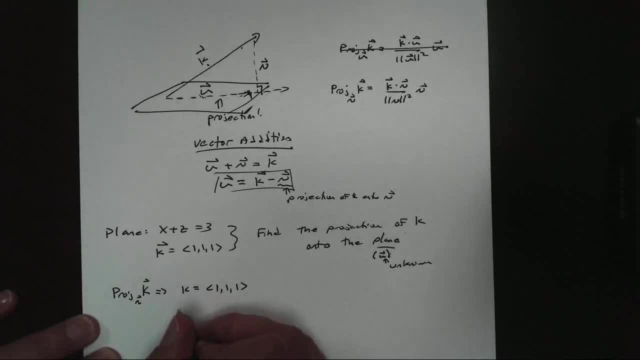 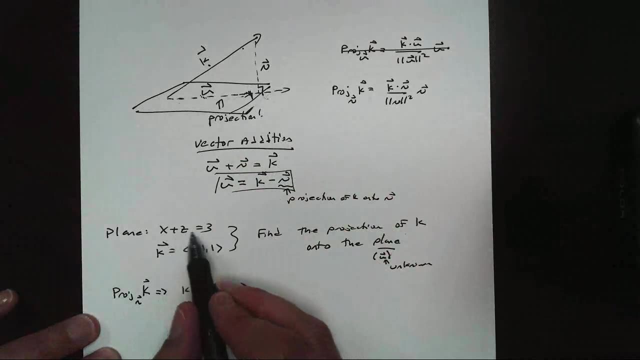 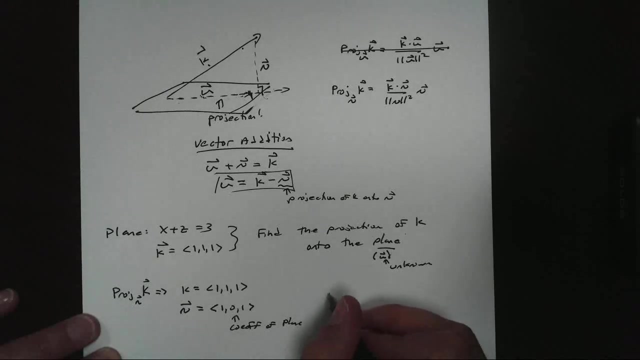 We also need the normal vector. Remember, the normal vector comes from the plane itself. If you know the equation of the plane, which we do, the normal vector just comes from its coefficients, That's the coefficients of the plane. To get my projection of: 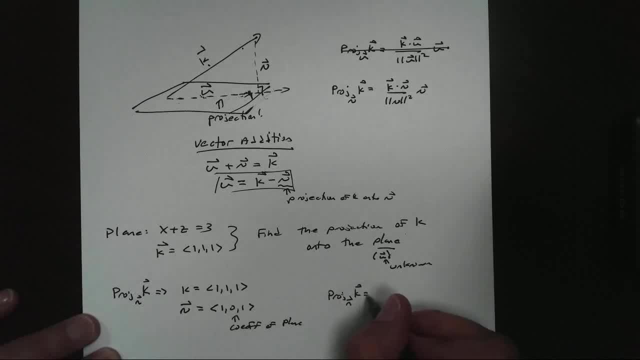 of k onto my normal vector. we just use that dot product 1, 1, 1,. dot that with 1, 0, 1, divided by the normal vector. the normal vector squared times the normal vector itself.